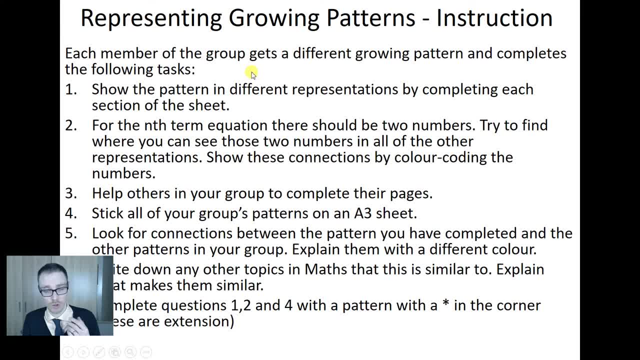 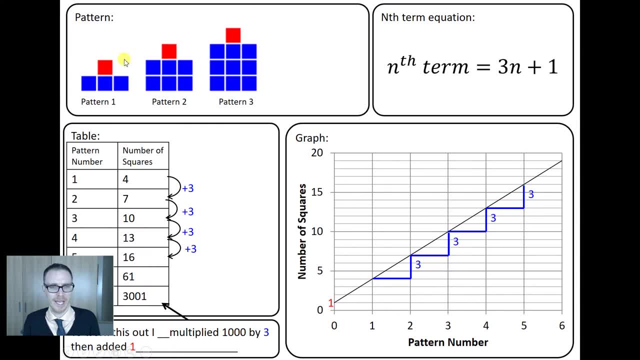 that's a lot of fun. It's a lovely way of doing it. There's nothing wrong, by the way, with kids just working through these independently or in pairs and so on. so just bear that in mind as we look through this So little worked example here and which will really kind of help explain what's going on. 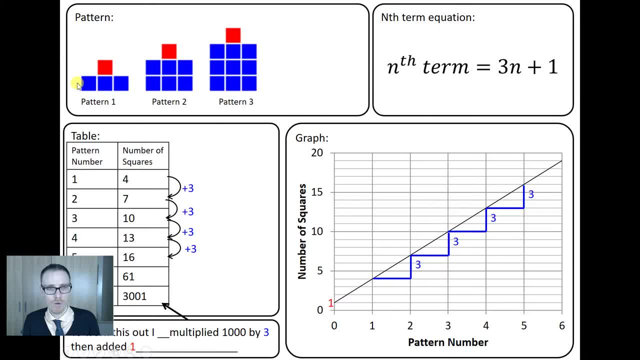 So every single sequence gets a visual representation and these are uncolored or not colored in, I don't know what the phrase is for that. when you see the, when you see them on the actual examples, then you get an nth term equation and then this is nice, then you get the table to see. 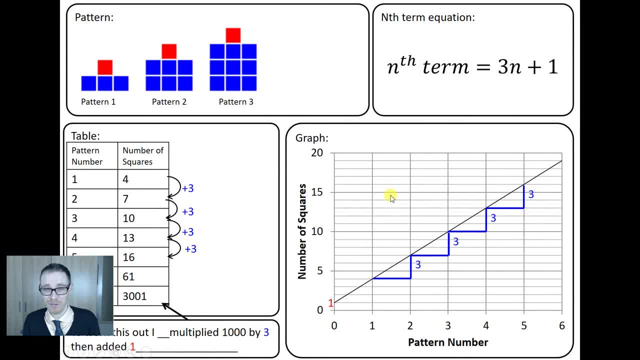 how they're growing. then you get the graph, because how often do we do that often, certainly, from a personal perspective, I very rarely relate graphs to sequences, but it's all the same thing, it's all related. and then, if I just move my annoying head out the way, a nice little sentence to work out. 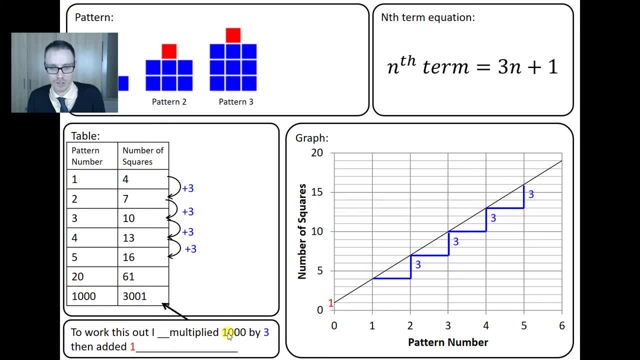 how many patterns, how many blocks in pattern? a thousand. I multiplied a thousand by three and added one, and so on. so four different things, four key skills- well, five. I guess that you can get From one a pattern representation, and then there's a load of these. so if I just move through these, 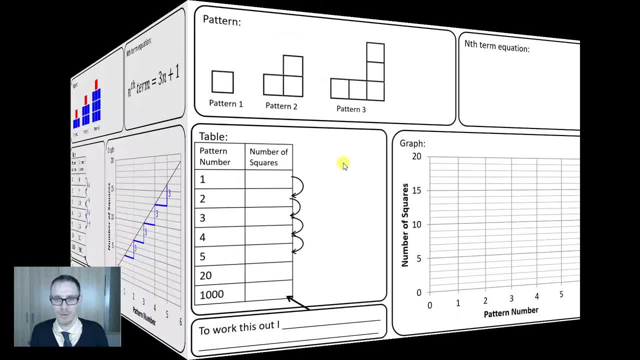 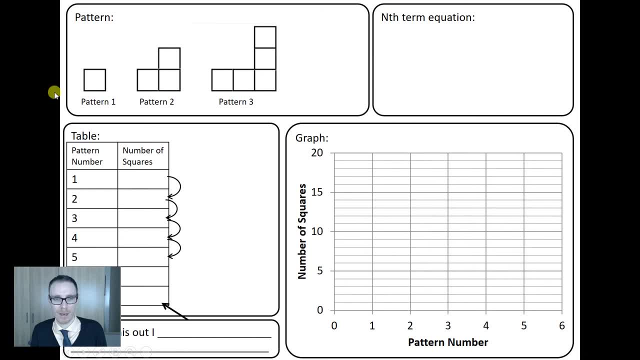 now. so let me just come. sorry, I clicked off. there we go, if I come through that now. so you get loads of these patterns. so kids will be given that pattern. they'll be asked to perhaps color in to see what stays the same, what's constant throughout it, what changes throughout it. therefore, what's the? 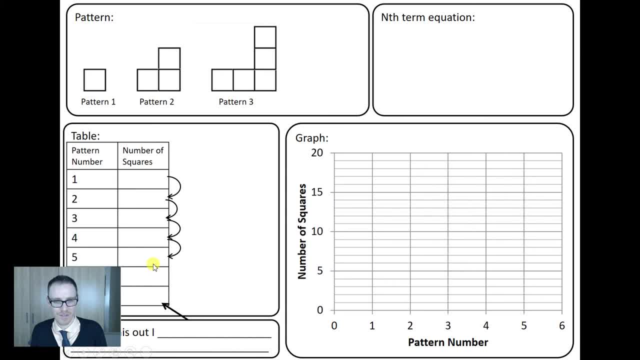 m term equation, and can they use that to fill out the number of squares? where does the graph come in to play? and then how would they work out the sat thousandth? and it'll be interesting to see which, which bits of this the kids find the easiest: what comes first, what comes second, and so on. 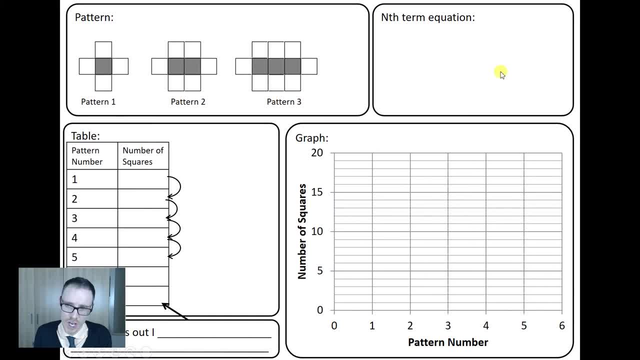 so again, coloring: what stays the same, what changes. where do the numbers appear in that m term equation? and sorry, that was something I really wanted to emphasize on here. it's a lovely thing. where does that three appear in each of these representations? where does that one appear? 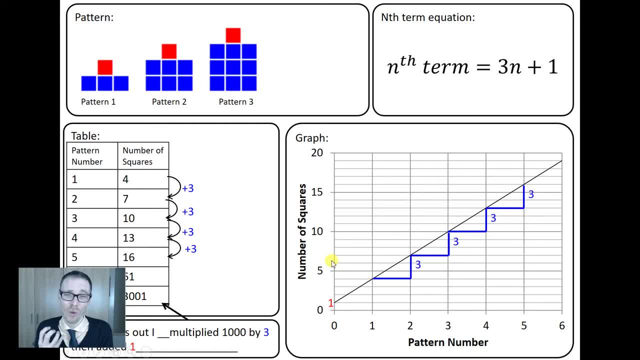 in each of these representations really nice, and it just gets kids to understand much more what this, what sequences, are all about. so, yeah, there's loads of these, loads of different ones, and as we go through then we'll see that all of these are linear sequences. but what I love about 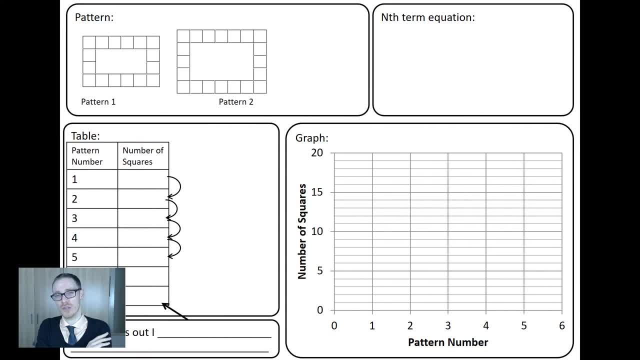 this is that this approach- and this is the same when you use any kind of picture approach- it lends itself perfectly well to bringing in quadratics without it seeming seen like a massive jump in understanding for the kids. so if I just go a little bit further, you can see the complexity increasing. 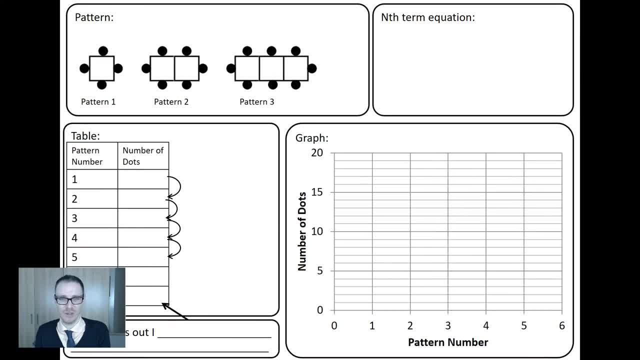 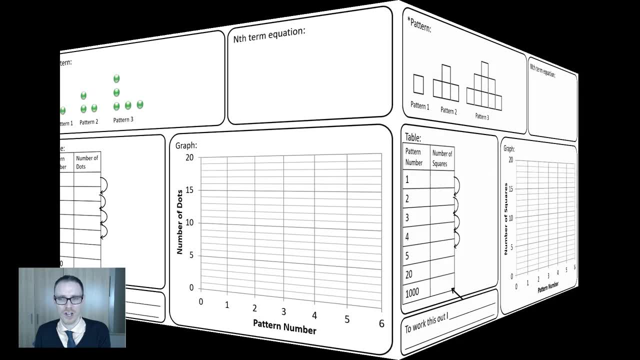 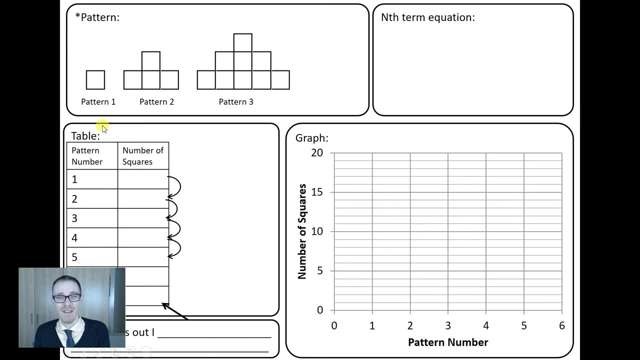 a little bit as we go through this and classic little chairs with tables around it and representation there. but as we get a little bit further, then we're going to start to get again. look at that pattern, what's going on there. so that will be an example of something that, if you didn't have this diagrammatic approach, that's. 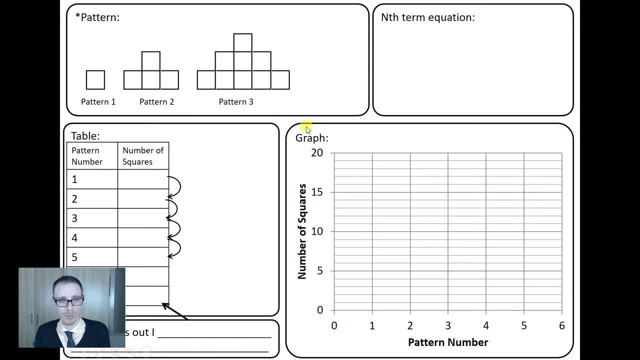 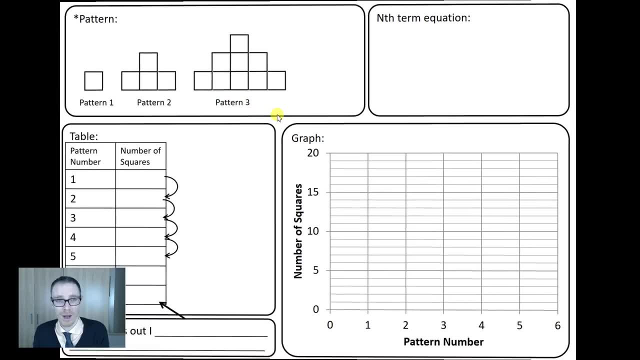 going to be incredibly difficult for the students, but I reckon they could probably have a go at that. it's got an asterisk by because it's a difficult one, but if you've kind of built them up through all these ones, maybe they're going to be all right with that, or at least they'll have a go. and again, 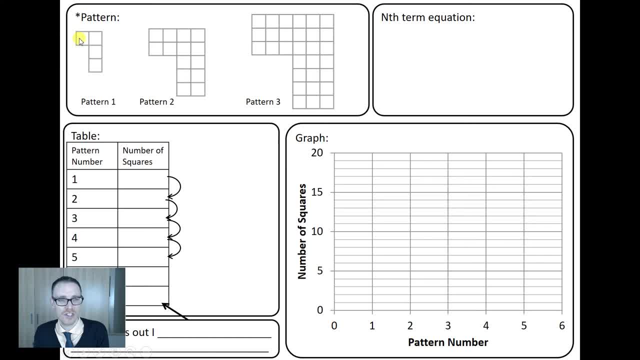 the quadratics start to come into play. but if students can start to see that as a single square that has kind of bigger square- two by two square and that was a three by three square- then they can start to build it up and it does, without having to fall back on the kind of quite tricky algorithm. 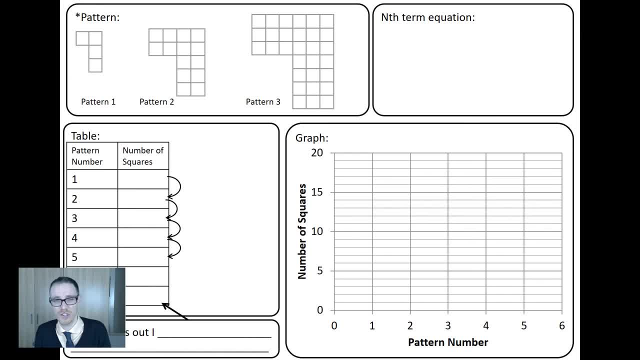 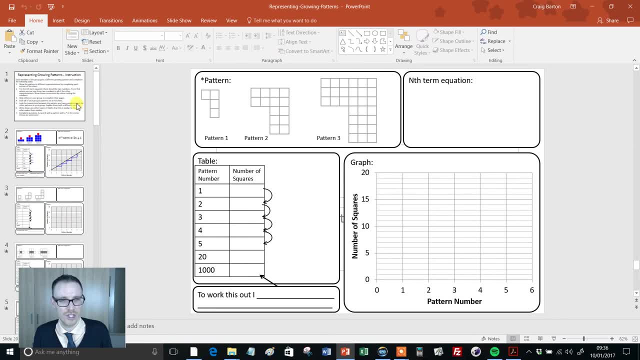 to work out the nth term of a quadratic sequence using second differences and all that kind of stuff. so look, I'm obviously incredibly biased because I've been looking into this research for years and this, this approach, but I've been doing this research for years and I've been doing this research for years and I've been 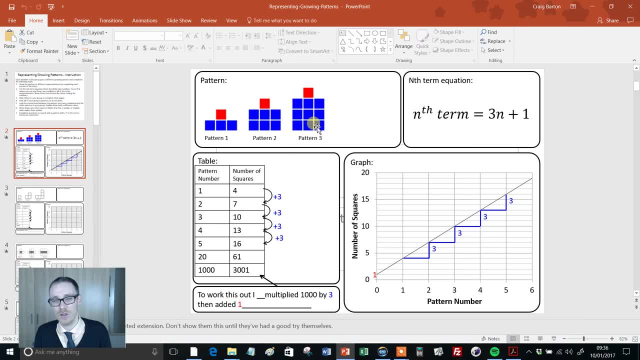 teaching sequences through a diagrammatic approach is. it has been shown to be a really solid way of doing it. and now, if you can use this resource to link it to the graphs, link it to patterns of numbers, it's just a complete package. so I just thought this was an absolutely sensational. 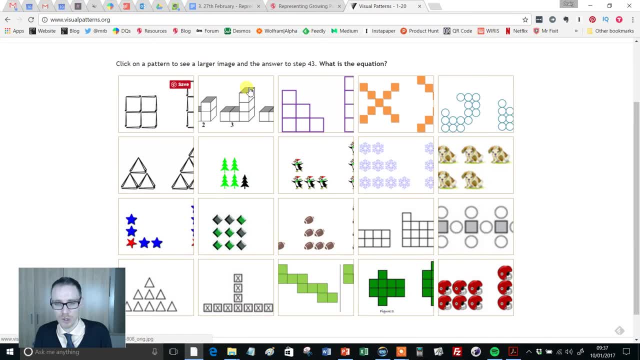 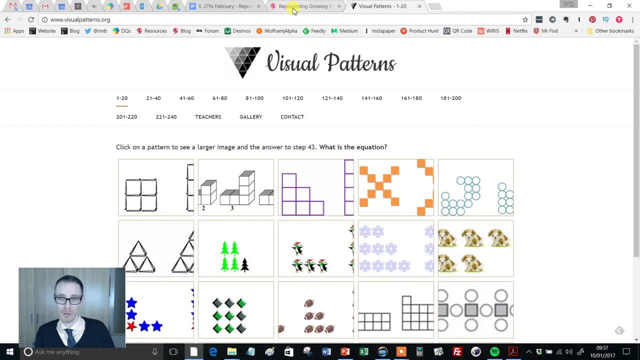 resource and I'd use it with any year group. you know I would use it any time I'm introducing sequences and this visual patterns. I've used this in primary schools with kids as young as kind of a teenager, so I'm not using the algebra, but who cares about that? that's not the important bit. 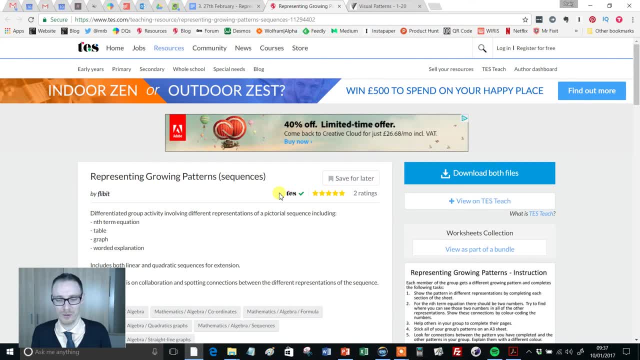 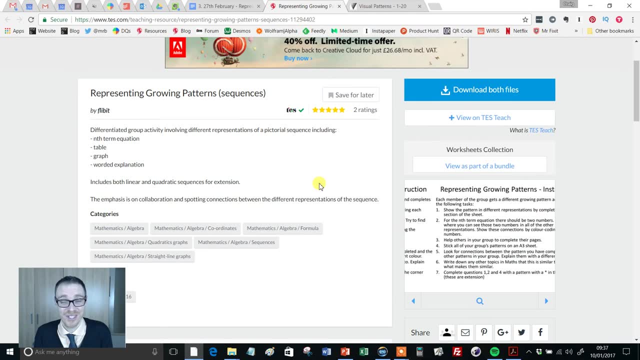 about it. so look, a wonderful, wonderful, wonderful resource. I hope you find it useful. I'd use it with anyone from year seven right up to year 11.. and yeah, and that's just about all I've got to say about it. so I hope you found that useful. if you like the resource, hop back onto this page and 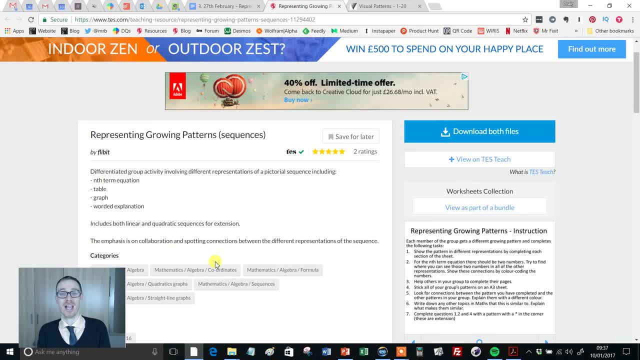 just share your thanks with the resource author and I'll return with a fresh resource the week next week. take care of yourselves. bye for now.